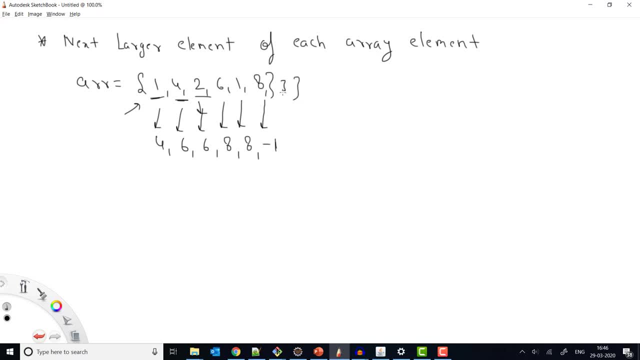 let's say, if it was one more element, three here, right. let's say, if it was three here as well, now if it is three. now if you see, for eight, for eight there is no such large element. even we have three, but three is smaller than eight. so in this case also we'll print minus one, because 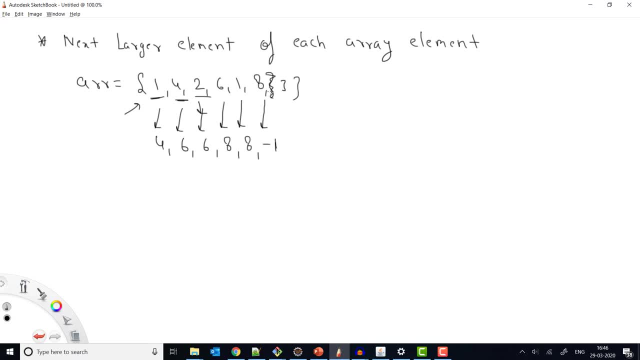 there is no such greater element. there is no such larger element for eight right now for the three, because we don't have any next element. so it will be minus one right. so basically, for each la value we need to print the next larger element present in the array right. 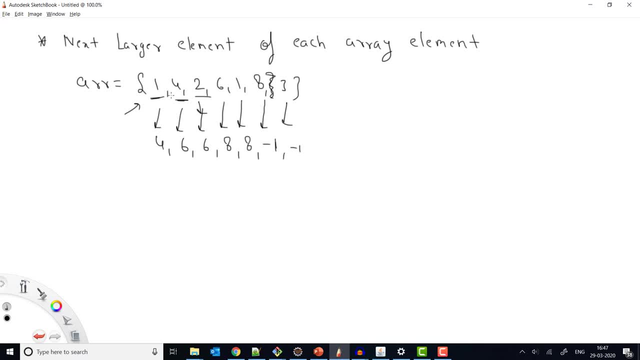 so we'll see one by one that how we can solve this question. then we will see the code of this and then we'll see the time complexity and space complexity to solve this question right. so now we'll solve this question using a stack. so first of all, take a stack, right. 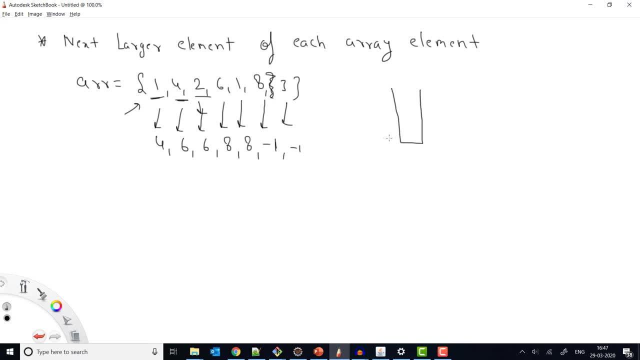 we'll take a stack and we'll and we'll push the first value into this one. this is the first value. now here we have one. now what i will do, i'll basically iterate from now. basically i'll iterate from: i equals to first index means the second value from here to the i less than area dot length. 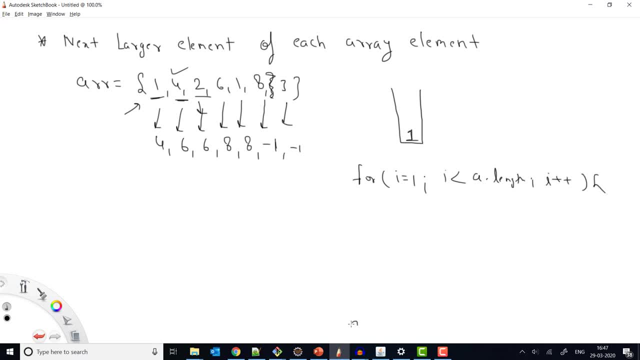 right now you will understand that, how. what we'll do now check with this one: that if this value, if the, if this four, if current value is less than the, the peak of this stack, so if this value is less than, it means this value cannot be the greater than this one. so it means, let's say, 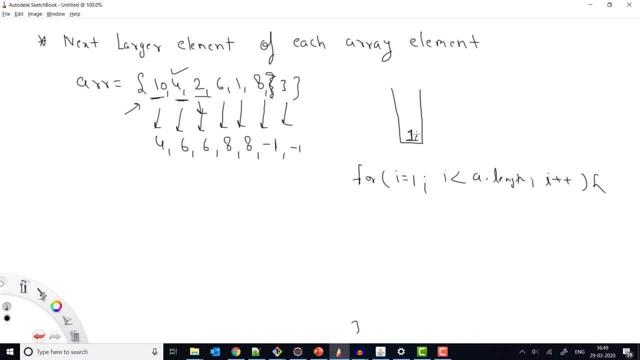 let's say, if it was 10 here. let's say, if it was 10 here, so we would have put 10 right now. check four. so if four is less than 10, if four is less than 10, it means four cannot be greater than this one. so if it is the case, we'll just put the four as it is in the stack. 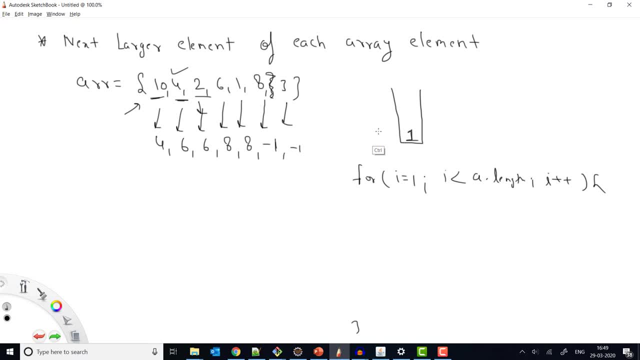 right. but let's say, if this value, the current value, is greater than the, the value which is present in the stack, it means this value is greater than this one. so if this greater than this one, it means we can say: for this value, this is the greater element it means. 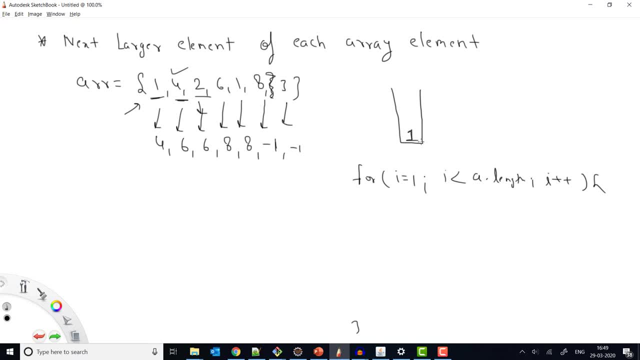 we'll print this value as the next greater element for this one. right, so now let's do that. so four is greater than this one. it means i will print four here and then i will remove this one because this is a greater element. so i it means this is done, i will remove this and i will push this four here. 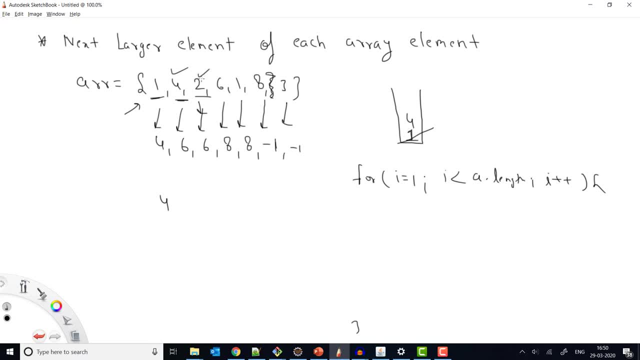 right now. let's check for the next element, for the two now, because two- and this is peak element, so 2- is less than 4. so if 2 is less than 4, it means i need to put 2 here. i won't do anything, i will just push the element 2 here now. check with this 6, now this 6. 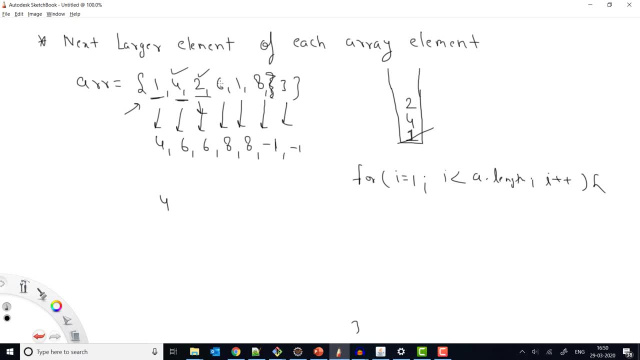 value is greater than 2. right, it means 6 is great. 6 is 6 is next larger element of this 2 right, so i'll remove the value from here and i will print 6 here right now. check for this 4 as well. now 6 is greater than 4 as well, so 6 will also be the next larger element for this 4 and. 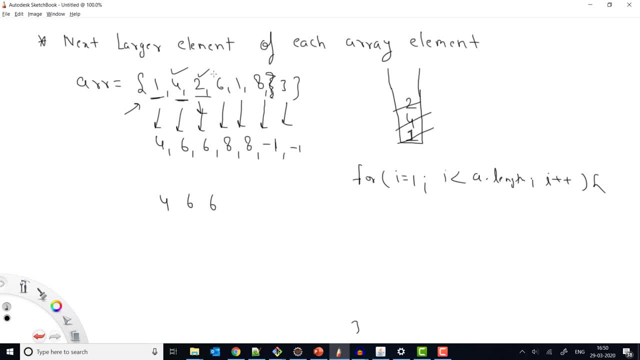 we will remove from here, right? so it means, if you see this 6 is both greater than the 4 and the 2, right, we can see from here as well, the 6 would be greater than the 6 and 6. so basically this thing. 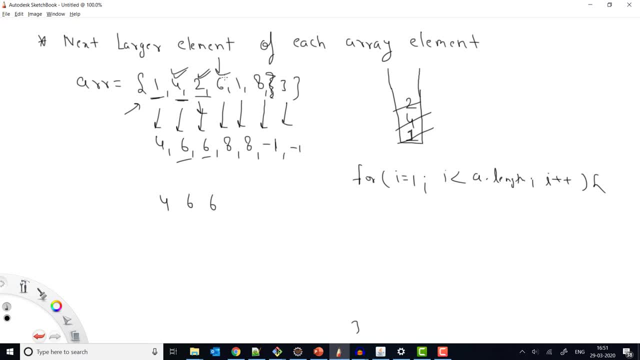 we need to do in while loop that we need to check the current value for all the values which are present in stack. so once you have checked this one, then we'll push this value 6 into stack. right now the next value is 1, so the next value is 1. it means 1 is less than 6. 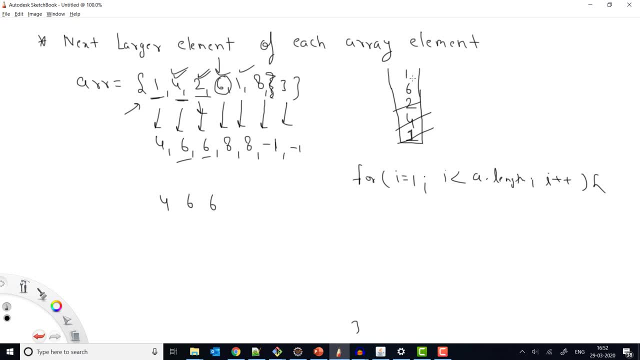 so if 1 is less than 6, it means we'll just push the value here right now. check with the next value, 8. now, 8 is greater than 1. it means 8 is the next larger element of this 1, so i will remove from. 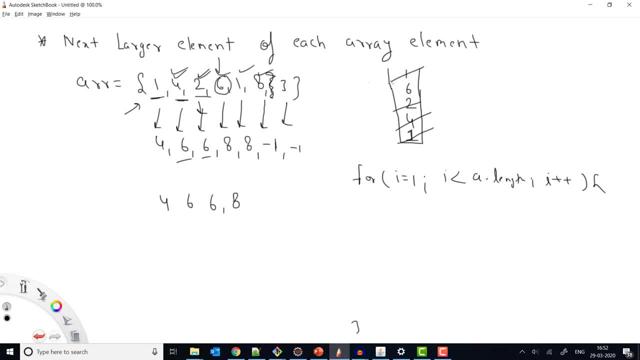 here and i will print 8 here now check. now check with the next element. now 8 is greater than 6 as well, so i will remove from here and i will print 8 because this is a greater element. now there is no such value, so i will push 8 here right now. the next element is 3. so if next element is 3 and 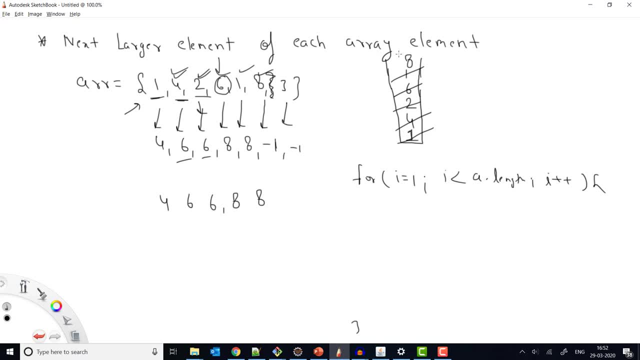 check: if 3 is greater than 3 is less than 8. so if 3 is less than 8, it means it means we'll just push the value here in the stack. so this is a stack, so we'll push 3 here right. so now there is no such. 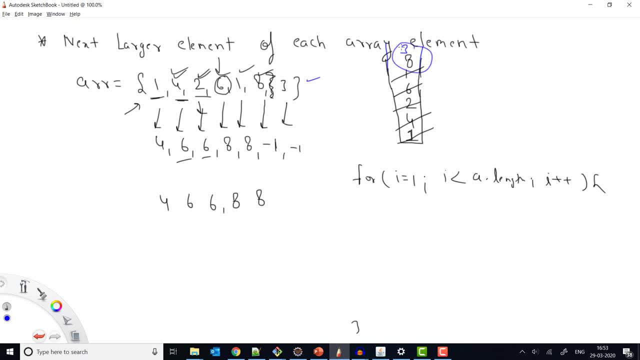 element here now. whatever element left in the stack will just pop out and will print minus 1, because for them there is no such greater value. so we'll remove minus 3. we'll remove 3 and we'll print minus 1. we'll remove 8 and we'll print minus 1. 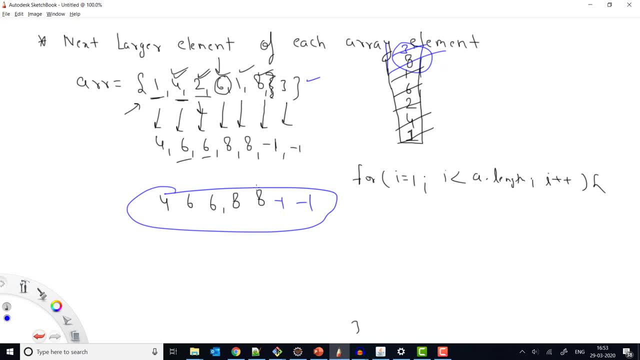 right. so you can see, this is a solution that we have done. now let's write the code as it is what what we have done? so, first of all, what we are saying, that for any value, we check that if, while if stack is not empty is empty. this is the first case. 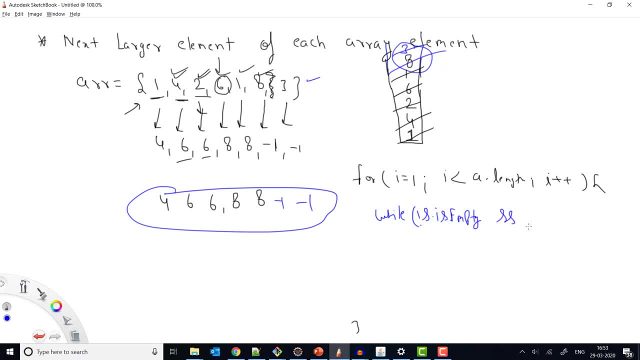 so stack is not empty. and we check that if the current value, if ai, is greater than the peak value, right, so if it is a case. so it means if, though, if two conditions are matching, that if stack should not be empty and if this value is greater than the peak value. so if this value is greater than 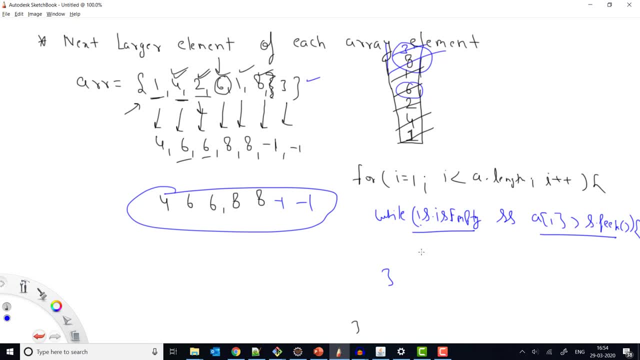 the peak value. it means this is the next greater element, this one. so in this case we print. we print element, because this is the thing. now we'll pop the value here as well. so basically, we'll pop the value from here, right? so this will happen until a stake is not empty and your value is greater. 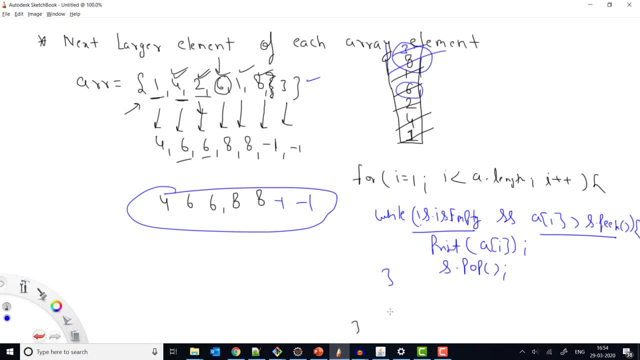 than the peak value, and after that we'll just push the value. so if it is greater than, then we do this. otherwise, what we do, we just push the value. after it will push the value right. so, whether this is greater than or less than once we, if this value is greater than, then we do this. 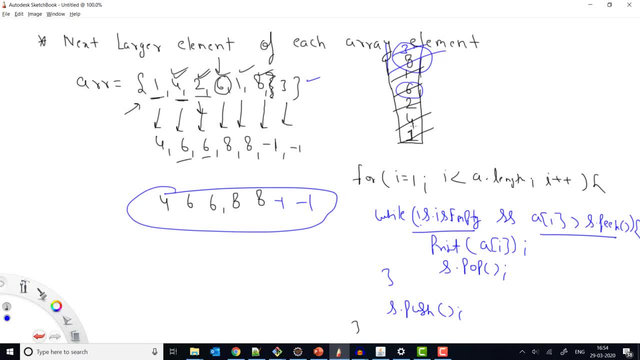 then then after doing operation, we push the value, and if the value is less than also, then also we push the value after that, right? so this is how we basically operate on this one right now, if you talk about the time complexity to solve this question. so basically, if there are n elements, 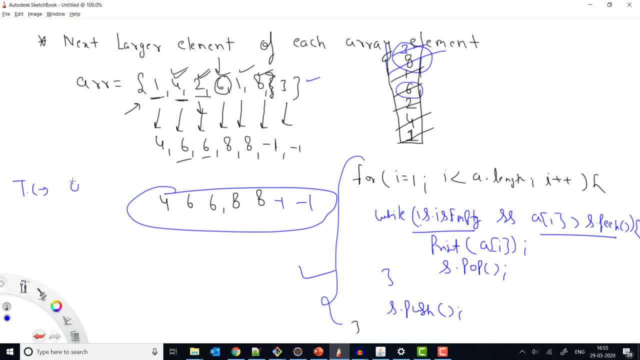 we are traversing basically all n elements, right? so my time complexity will be big of n. and if you talk about the space complexity, so because we are taking a stake. so at maximum we need to store the n values. so my space complexity will also be big of n. right now let me show you the code as well. 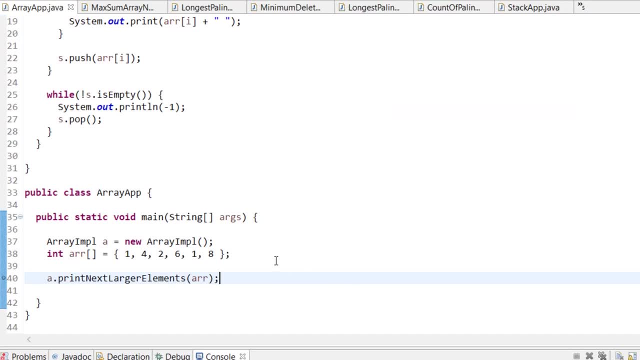 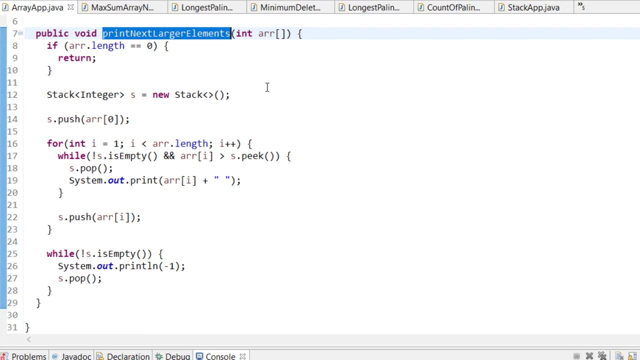 so that you can get it better. so here we have an array and here i am calling the function print, next larger element where i am passing the array. so now these are the. this is the basic case, that if my array length is zero, it means i don't have any elements. in this case i will return, i won't. 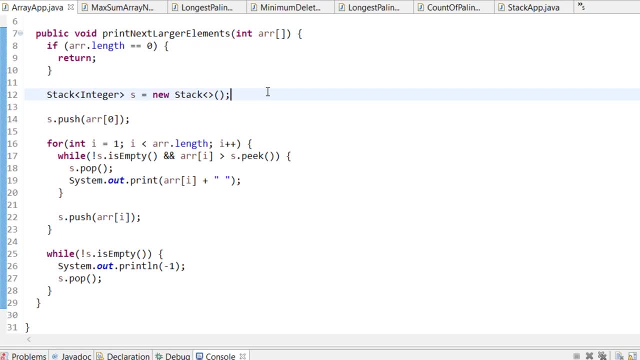 print anything. otherwise i take a stack of the integer values and i push the first value. now what i do? i basically start from the i equal to 1th index and till the array length and i check that if my array, if my stack is not empty and if the array element is greater than. 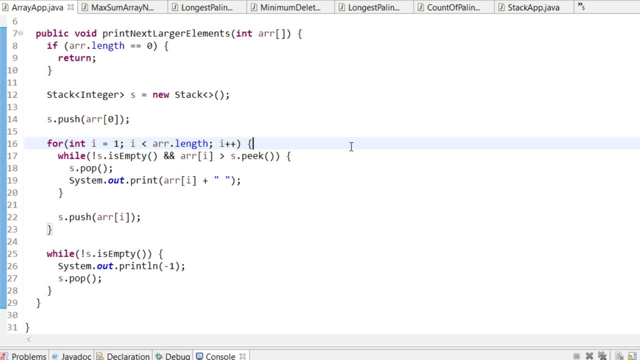 the peak element of the stack, then what you do? you basically pop the element and you print the current value, because the current value is larger element of the of the stack. what is the peak value? right? so you do this in the while because there can be many element, and then after that you push the current value in the stack, right? so once you do, 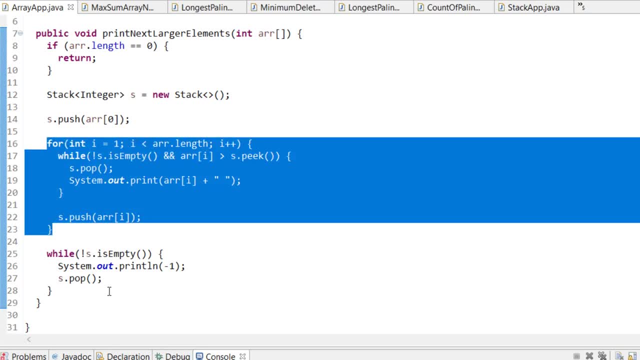 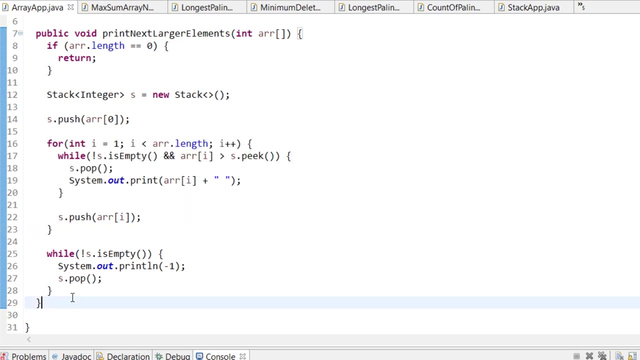 that this is. once you are done with this one, then whatever element left in the stack- so until stack is not empty, you basically print minus one. because what for whatever values are remaining in the stack, for that there is no such larger element. so we'll print minus one, right? so this is how. 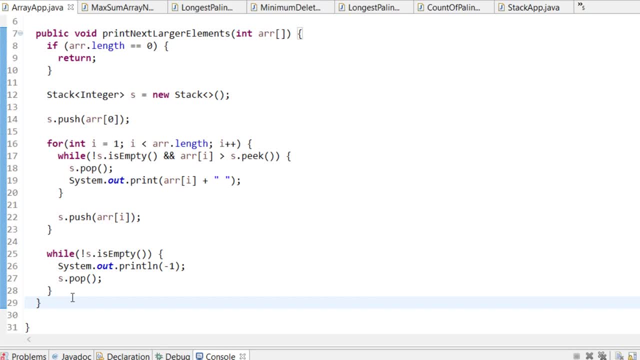 we can basically print the next larger element of each array value, right, so that's it, and if you have any doubts regarding this, please write in the comment section and i will also push the source code into description section, so if you want, then you can also get it.